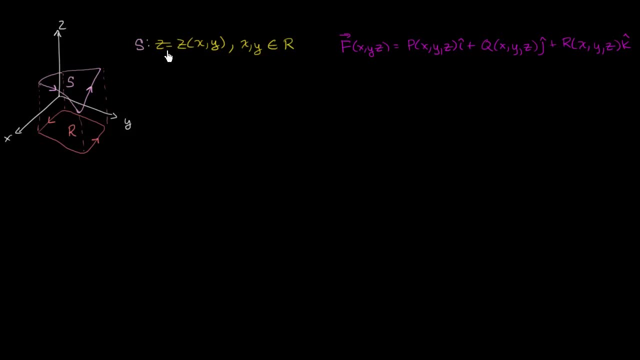 The other thing that we are going to assume that z, which is essentially a function of x and y, that this function of x and y has continuous second order derivatives, So continuous second derivatives, And the reason why I'm going to make that assumption. 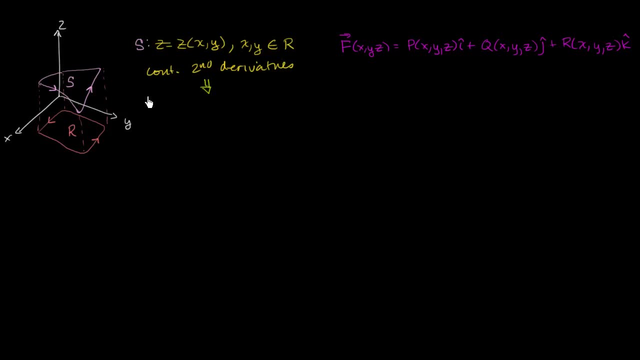 is. it's going to help us in our proof later on. It's going to allow us to say that the partial of our surface, or the partial of z with respect to x, and then taking the derivative of that with respect to y, is going to be the same as the partial of z with respect to y. 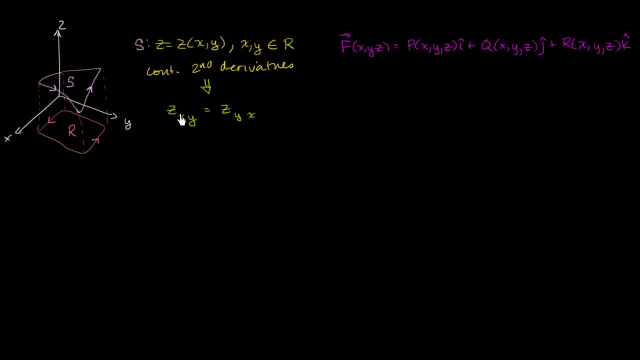 and then taking the derivative of that with respect to x. And in order to be able to make this statement, we have to assume that z, or this z right over here, z is a function of x and y has continuous second order derivatives. 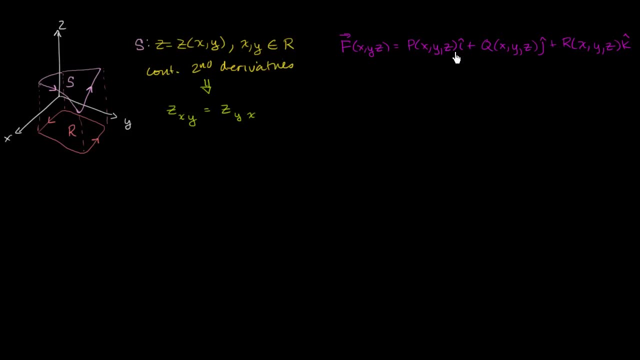 And over here we've just written our vector, field f, that we're going to deal with when we're trying to play with Stokes' theorem, And we'll assume that it has continuous first order derivatives. Now, with that out of the way, let's 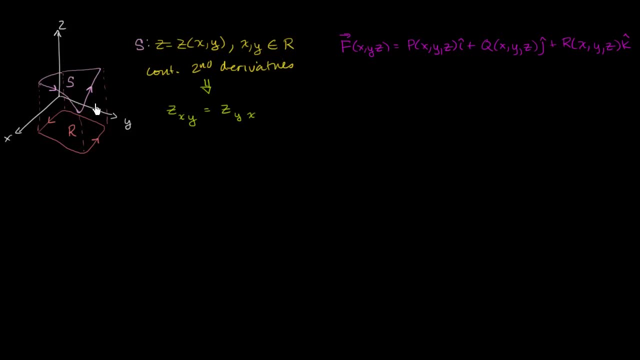 think about what Stokes' theorem tells us, And then we'll think about, for this particular case, how we can write it out, And then hopefully we will be able to do that. And then hopefully we will be able to do that. 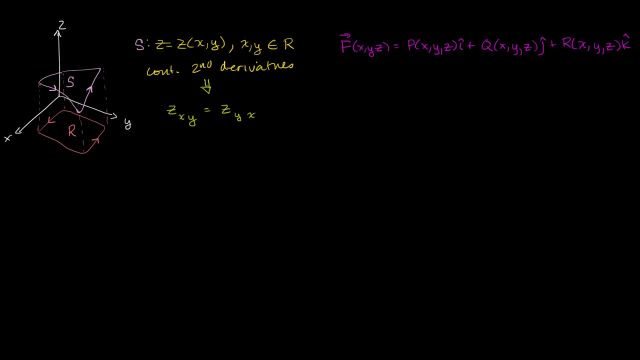 And then, hopefully, we will see that the two things are equal. So let me write it out. So Stokes' theorem tells us that f dot dr over some path, and the path that we care about is essentially this path right over here. I'll do it in blue. 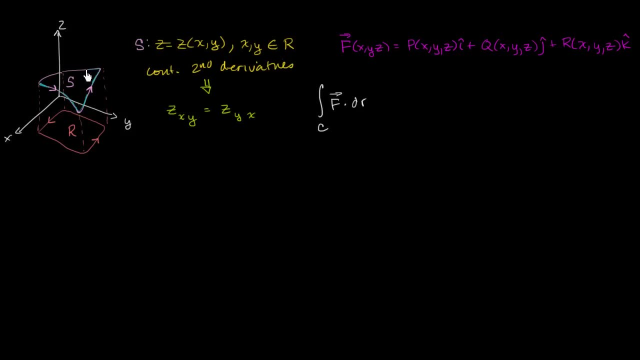 It's this path right over here. This is the boundary of our surface, So this is c right over here. Stokes' theorem tells us that this should be the same thing as this. This should be equivalent to the surface integral over our surface of curl of f dot ds. 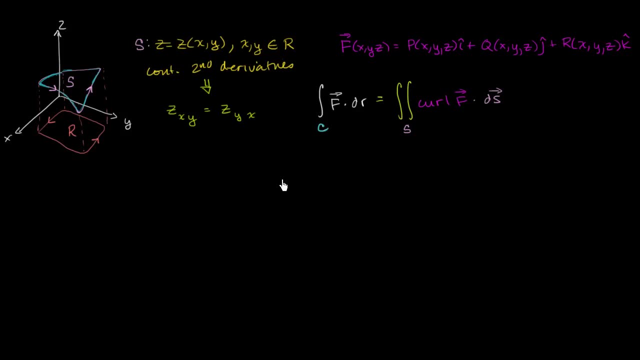 dotted with the surface itself. And so in this video I want to focus- or probably this and the next video, I want to focus- on the second half. I want to focus this, I want to see how we can express this, given the assumptions we've made. 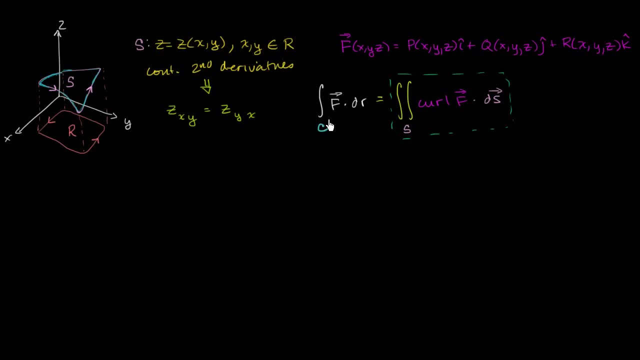 And then after that we're going to see how we can express this given the same assumptions, And then hopefully we'll find that we get them to be equal to each other. So let's just start figuring out what the curl of f is equal to.